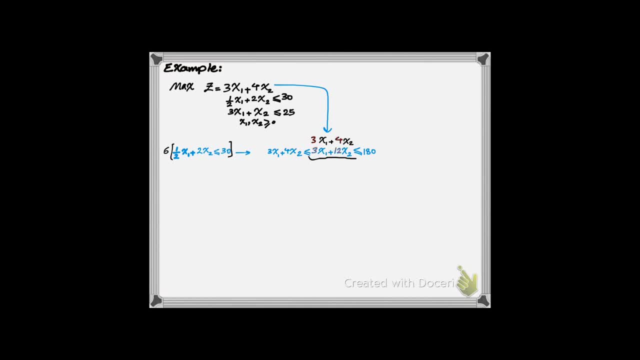 equal to my objective function. You can experiment that by plugging some values for x1 and x2.. For example, you can put 4 and 5 for the value of x1 and x2.. If I put 4 and 5 for the first term, I get. 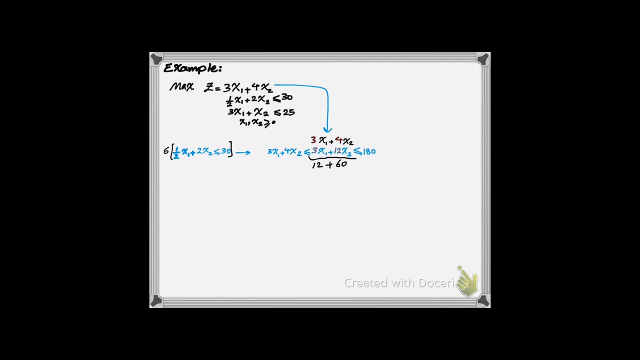 12 and for the second term 60. If I add them up, it's 72.. Now plug 4 and 5 here and you see the value. here that you get is 20 and here is 12, so you get 32.. So basically any value for x1 and x2. 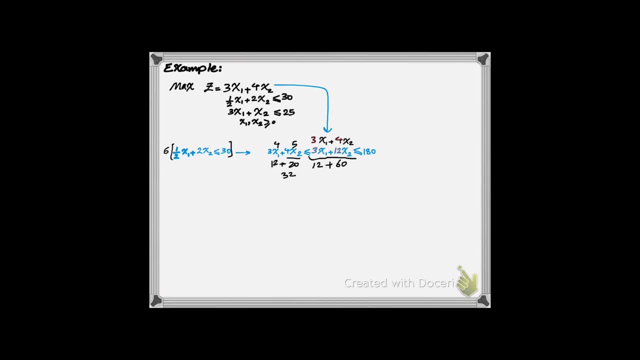 you plug in the second equation. this equation is going to be greater than this equation, and the reason for it is that the coefficient of x1 and x2 here are greater than their equivalent in the objective function. So you can conclude that objective function is less than or equal to 180.. 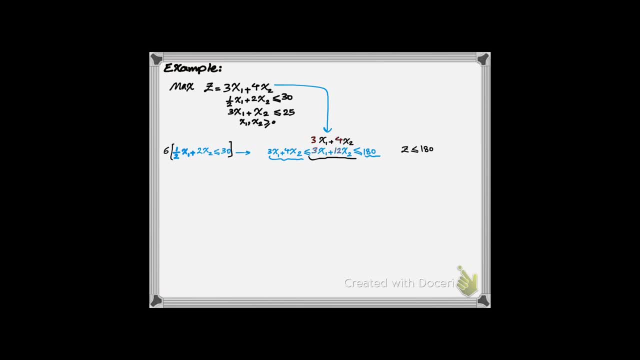 I can write this statement as z less than or equal to 180.. Now let's do the similar exercise with the second constraint of the problem. Now I'm going to take the second constraint and multiply it by 4 on both sides. So if I do that, the new constraint is going to be 12x1. 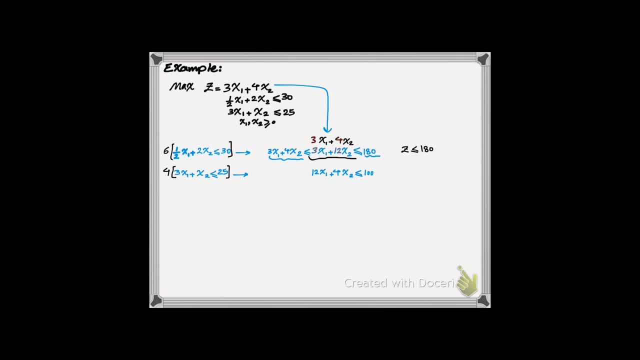 plus 4x2, less than or equal to 100.. Now compare the coefficient of x1 and x2 here with the coefficient of x1 and x2 in the objective function. Now what you see is that again, 12 is greater than 3 and 4 is greater than or equal to 4.. 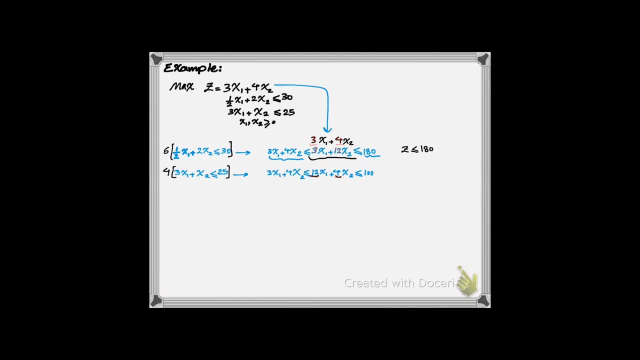 And, as a result, this term also is greater than or equal to your objective function. So I can write this as z less than or equal to 100.. Now notice that we are trying to maximize the objective function and now we know that the maximum of objective function cannot exceed 100, right? So if 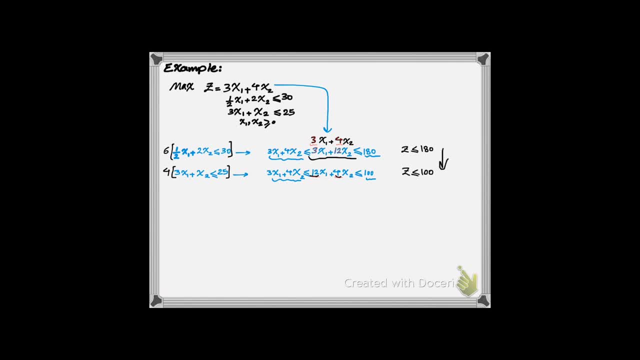 I find the minimum value that my objective function can grow to. basically, I can find a maximum value for my objective function. So now, as you see, this time we can approach the problem differently. We are trying to find to what extent we can reduce the right hand side of this constraint, because if you find that minimum value, 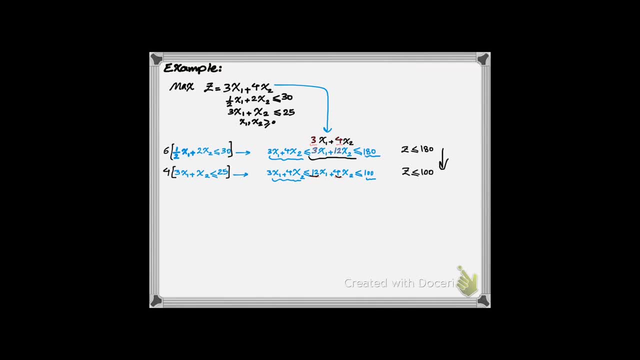 is equivalent to the maximum of our objective function. So to achieve that, let's this time take a look at a linear combination of the first and second constraint of the problem. So this time I multiply the first constraint by 2 and add it with the second constraint. 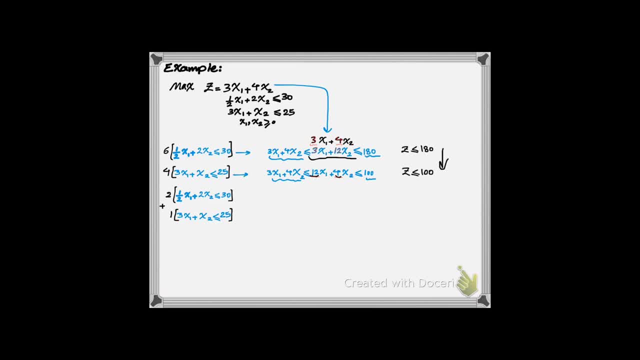 So mathematically there is no problem with doing that and the new constraint that we get is 4x1 plus 5x2 less than or equal to 85.. So to explain how this new constraint has been generated, you multiply 2 by x1, equal coefficient, which is 1 half, and you get 1x1. and from the second, 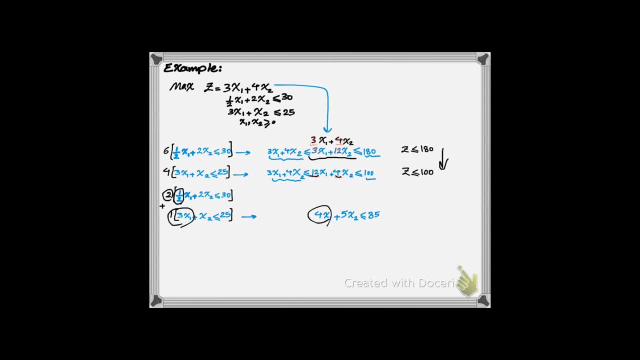 constraint. you get 3x1. you add these two up and you get 4x1.. Similarly, you can do apply that to the second variable. 2 multiply by 2 is 4x2 plus 1x2. you get 5x2. that provides this term, and if you, 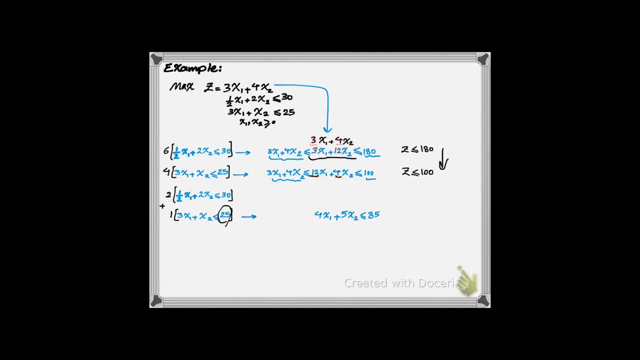 multiply 2 by 30, you get 60, and you add it by 25 and you get 85.. So that's how this new equation has been generated: It's a linear combination of these two constraints. Now, what you notice here again is: 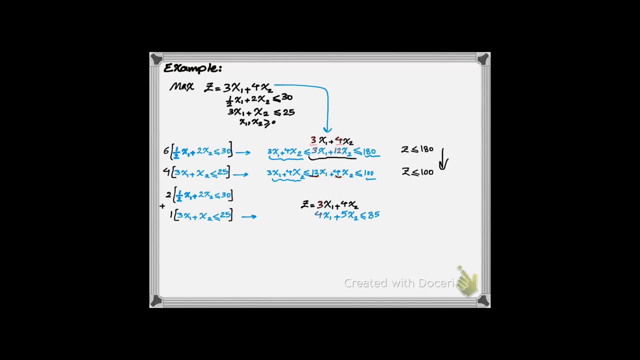 the coefficient of x1 and x2 are greater than their equivalent in the objective function, So 4 is greater than or equal to 3,, 5 is greater than or equal to 4, and then therefore this term is greater than the objective function, because any positive value of x1 and x2 that you put in this 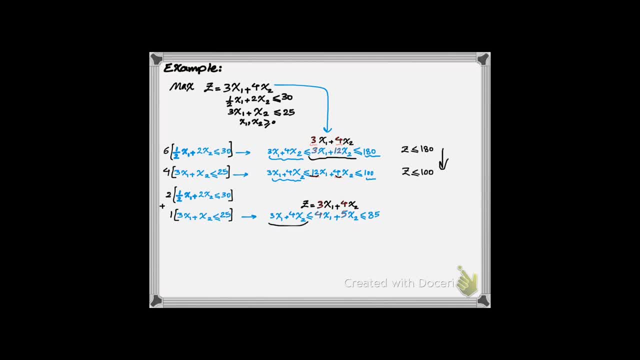 equation is going to give you a greater value than this equation. So therefore you can say z is less than or equal to 85. So if you're trying to maximize z, the value of z is not going to be anything more than 85, because mathematically it is not possible. 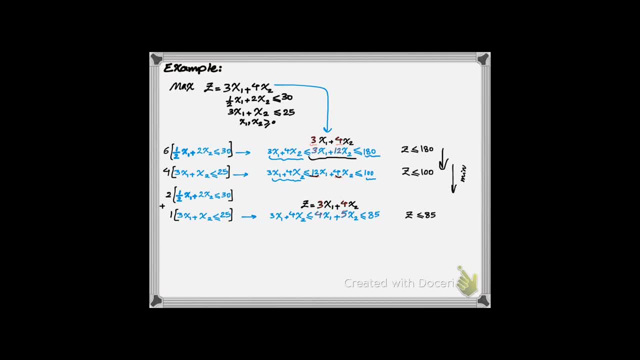 Now, as you see, if we minimize again this value, we can achieve to the maximum of z value. So the question is: what should we put instead of 2 and 1 so that it gives us the minimum value possible on the right hand side? So let's put y1 and y2 as unknown amounts that we can multiply by these. 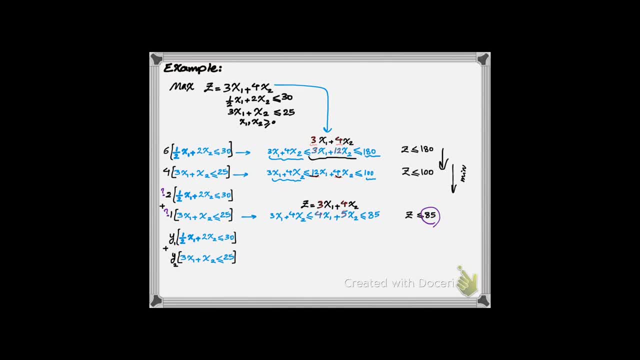 constraints so that we get the minimum value on the right hand side. So I'm going to put y1 and y2 as the multiplier, because these are the value that we want to determine. So if I do that, y1 multiplied by 1 half gives you 1 half y1 plus 3y2.. So that becomes the coefficient of x1, and then we 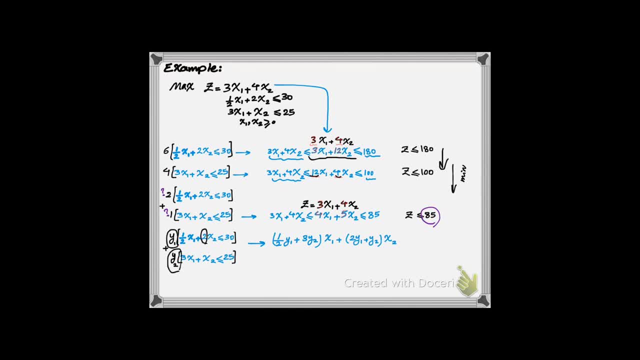 have y1 multiplied by 2 plus y2 multiplied by 1 as the coefficient of x2.. Now we want this whole term to be less than or equal to 30y1 plus 3y2.. So we're going to put y1 and y2 as unknown amounts. 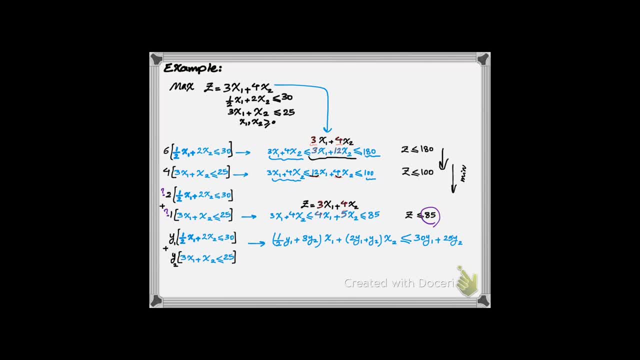 plus 25y2, which is the linear combination of these two constraints. However, what we are trying to do is to minimize this side. We have two conditions. First, we want to make sure that the coefficient of x1 is greater than or equal to 3 and coefficient of x2 is greater than or equal to 4.. So, basically, 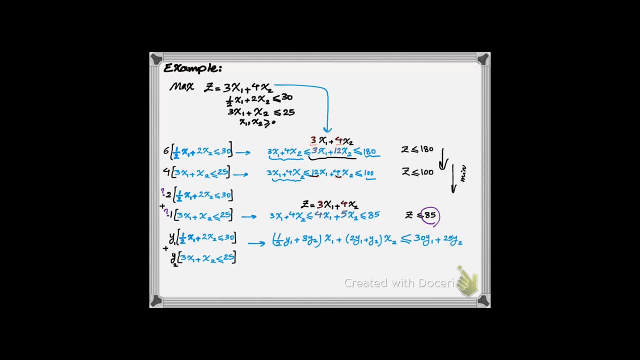 we're dealing with a new optimization problem with two constraints. Let's write that down. So it's going to be 1, half plus 3y2 should be greater than or equal to 3, which is the coefficient of objective function for x1. 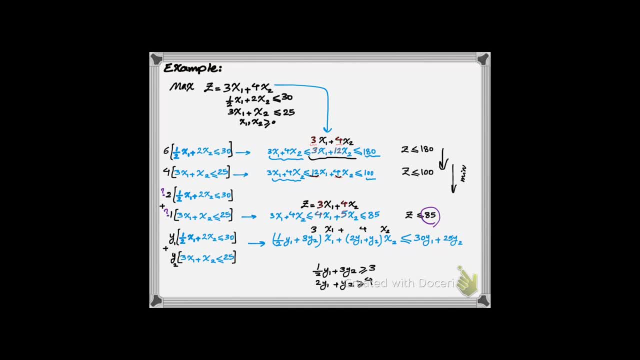 and the second condition is 2y1 plus y2 greater than or equal to 4, which is the second variable objective function in coefficient. Now we want to minimize the value of right hand side here, which is 30y1 plus 25y2.. So basically we achieve to a linear programming problem. the second problem: 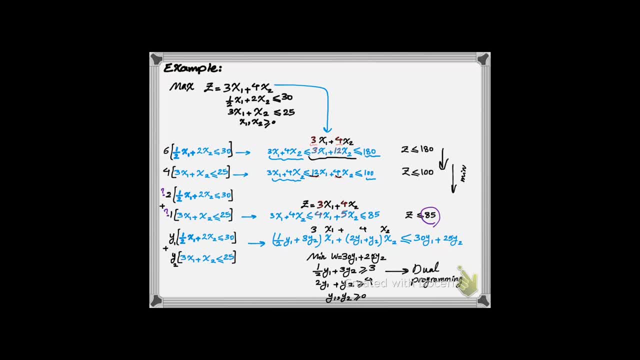 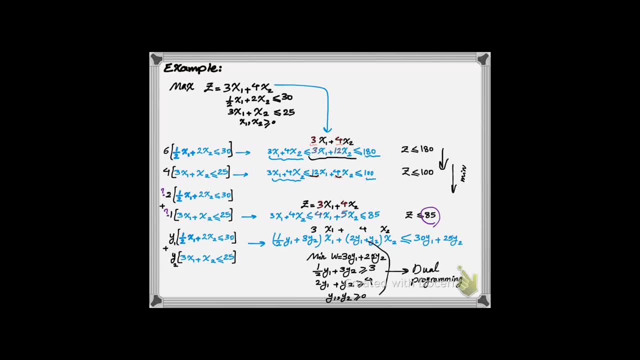 have a dual programming problem. In dual programming problem we're looking at the problem from a different perspective. We start from some upper bound and try to minimize that upper bound to get to the maximum value that z can grow. The relationship between dual and primal problem are very interesting. Let's look at the dual programming properties, The very first. 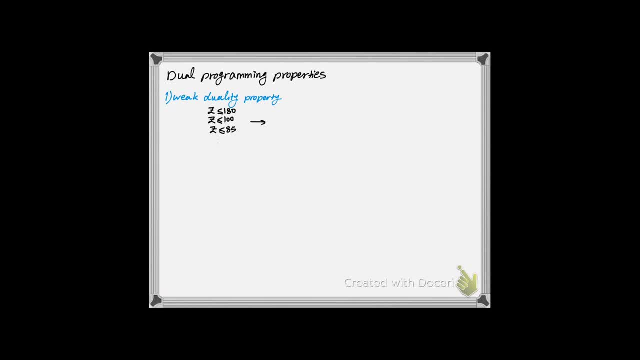 property that we're going to review is weak duality property. If you notice, we had z less than or equal to 180, z less than or equal to 100, z less than or equal to 85 and we keep creating upper bounds for the primal problem objective function. So the weak duality property is very related to that. 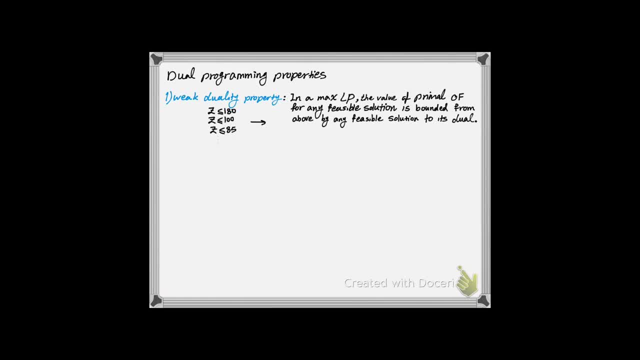 example that we saw, We can say in a maximum LP. we can say in a maximum LP, we can say in a maximum LP or in a maximization LP, the value of primal objective function for any feasible solution is bounded from above by any feasible solution to its dual. So if your dual programming problem, 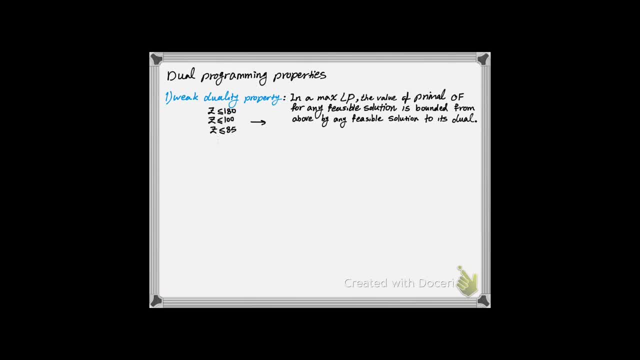 has a solution. its value is bounding the primal problem and create an upper bound for it. The same statement is true for a minimization problem. So in a minimization problem, the minimum amount is limited by a lower bound, what we call. So let's. 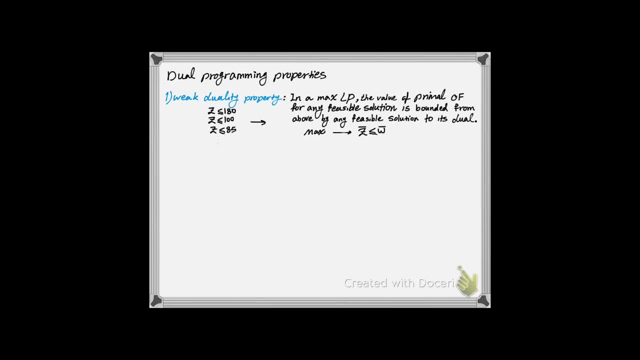 write this in a mathematical format. You can always say: the value of objective function for any feasible solution in the primal problem is less than its dual objective function for any feasible solution that is given Now for a minimization problem. this is going to be the 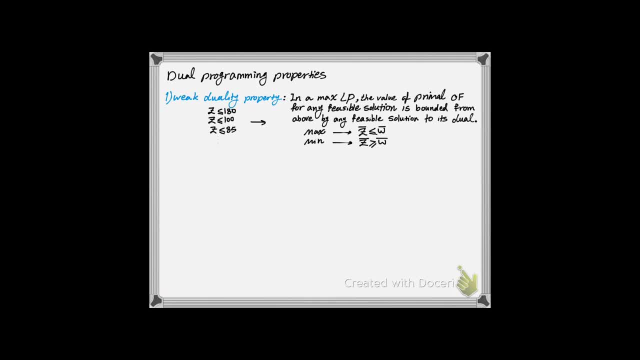 other way around. The value of a primal objective function for any feasible solution is bounded from below by any feasible solution to its dual. The second property is unboundness property. If primal problem has an unbounded solution, then the dual is going to be infeasible. 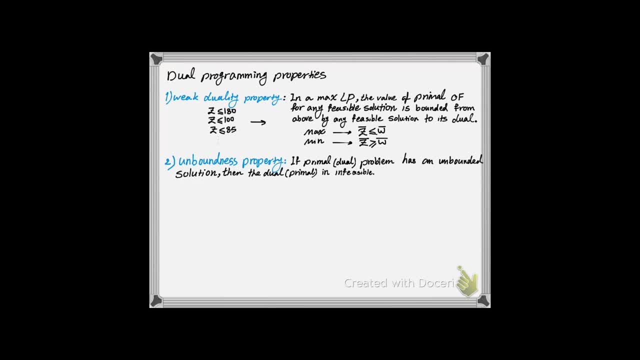 How. Let's explore this. This can be concluded from the first property, which is weak duality property, How We said that in a maximization problem we are bounded from the above by the feasible solution of its dual. Now suppose that your primal is unbounded. It means that it can. 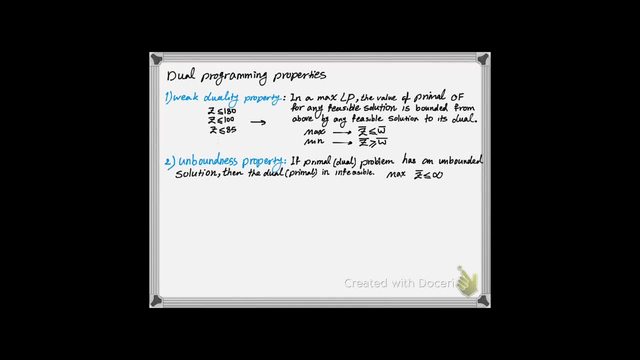 grow to infinity. Then the question would be: can you find a value for dual problem that makes this primal problem bound? The answer is no, because this is infinity. So you cannot really find a solution and plug into your dual that restricts that value. So the unboundness can be concluded from the weak duality property.